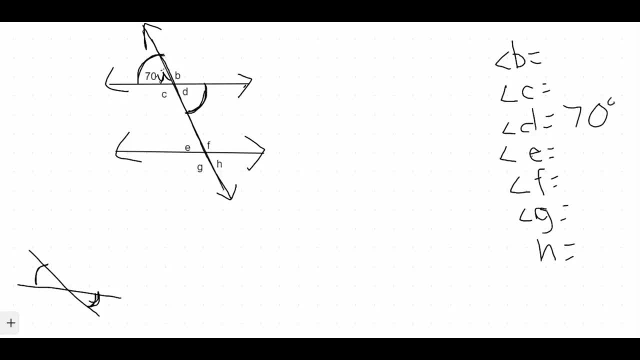 So if angle B is angle D, which means D also has to be 70 degrees. What I can also do at this point here is I can use corresponding angles. Almost pretend, if you're looking at this top grouping of angles- angles A, B, C and D- almost pretend that you. 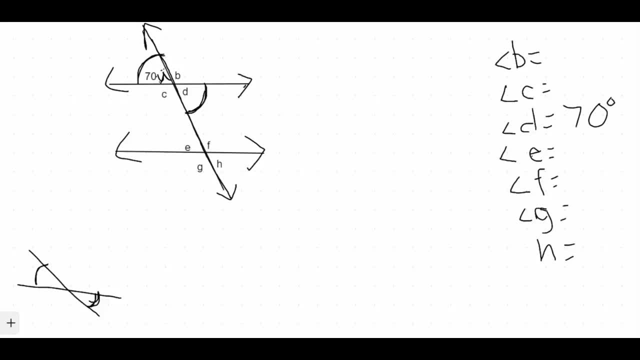 can pick up those four angles and set them right on top of the E, F, G, H, and what angles would match up with each other? A would match up with E, B would match up with F, C would match up with G and D would match up with H. 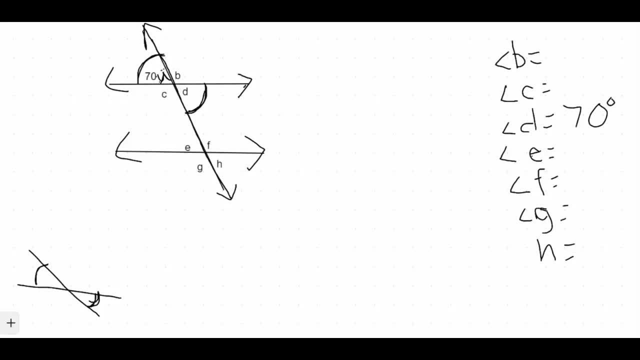 And what we know about corresponding angles is that corresponding angles are also congruent. They equal each other. So if angle A corresponds with angle E, that means those two would be the same, And since angle A is 70, angle E also has to be 70 degrees. 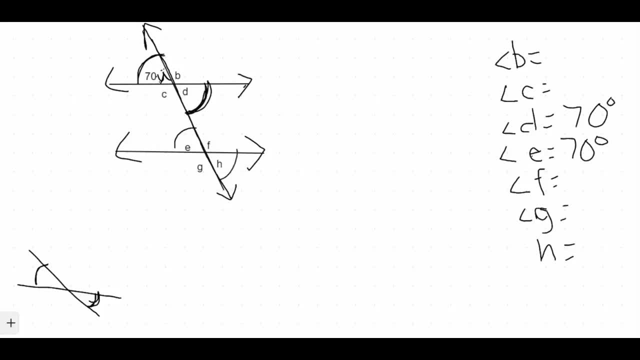 Same thing for D. That bottom right angle there would match up With the bottom right angle of H. so D and H would also be corresponding angles, And since D is 70 degrees, H also has to be 70 degrees. So what we're going to do here is we're going to use supplementary angles to then find our other missing pieces. 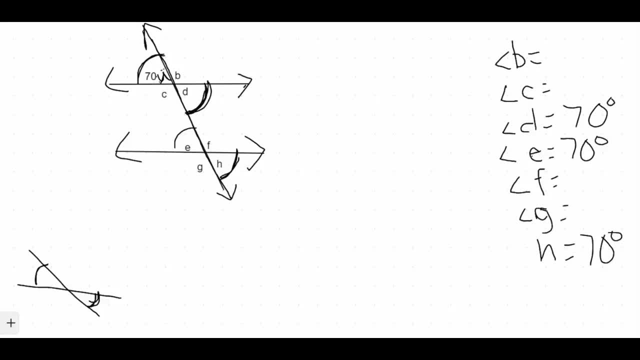 here. There are a few different ways that you can look at this problem here, but I'm going to use supplementary angles. So a supplementary angle looks like a straight line and a supplementary Angle equals 180 degrees right. It's half of a circle. 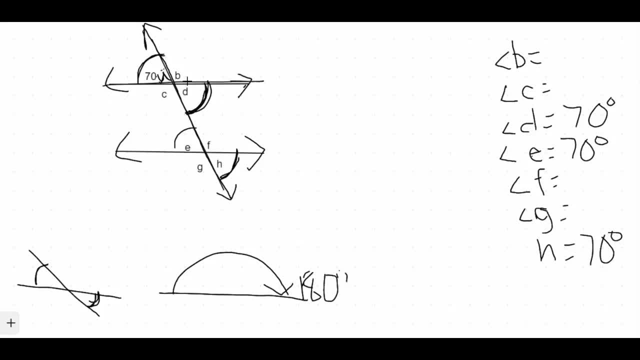 So I'm going to pick any straight line on this figure that I have here and I'm going to pick this top straight line there. And because it's a straight line, I know that this is a supplementary angle, So everything inside here has to equal 180 degrees. 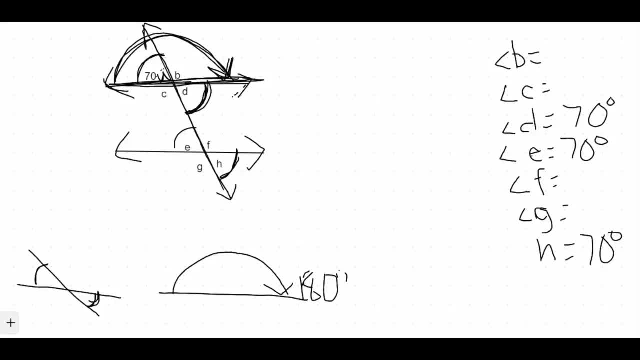 Now I know that angle A equals 70 degrees. So if all of this Here, if angle A and angle B make up a supplementary angle, that means angle A plus angle B have to equal 180 degrees. So if I take that 180 degrees and I subtract away angle A, it's going to leave me with angle B.